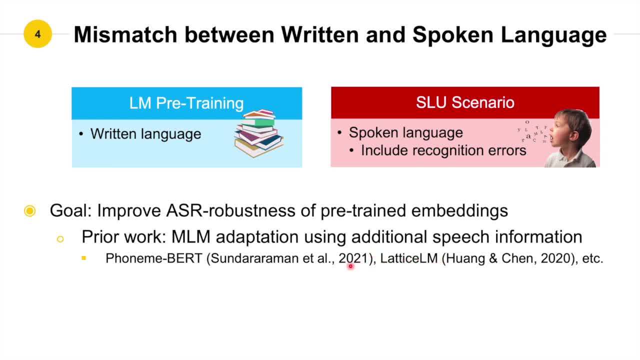 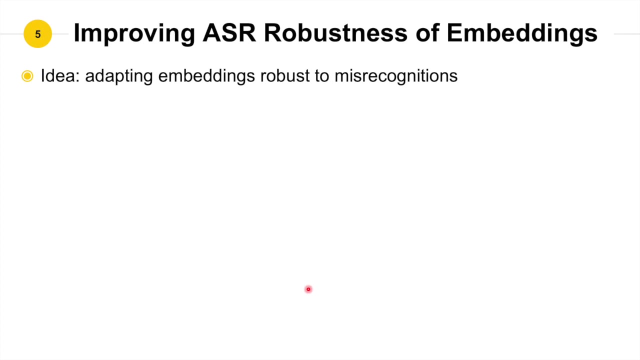 But the additional speech information is very difficult to collect at both training and serving time. Therefore, in this work we propose a new adaptation method using only textual information, And the idea is to tell the model about the correct text behind the erroneous ASR output. 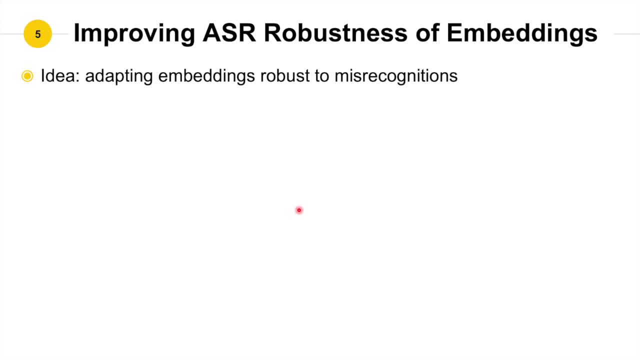 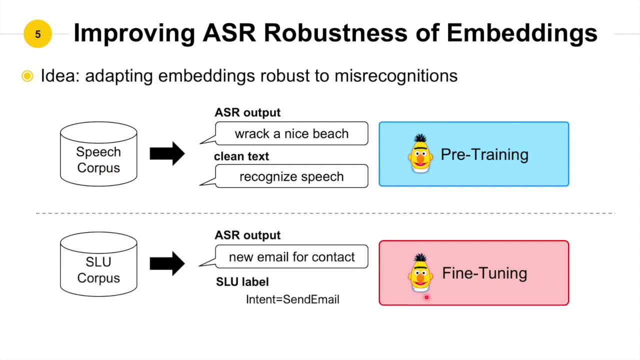 And our training strategies can be divided into two stages: The pre-training stage using a speech corpus and the fine-tuning stage with SLU corpus. Let's first look at the pre-training stage. We propose the contrastive pre-training for spoken scenarios. 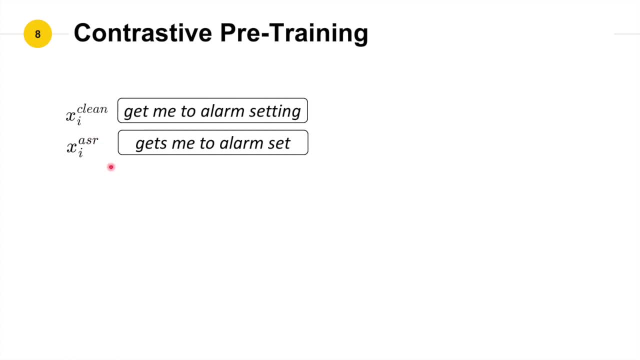 First we have to prepare the paired data. A positive pair is composed of the clean text and the ASR output of the same speech, And the idea is that we ask the model to pull closer the embedding of the two sentences so that when the model only sees the erroneous ASR output, it can infer the correct text. 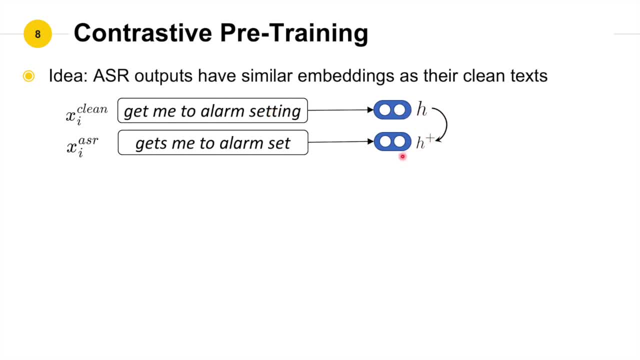 because their representation should be very close. We also collect negative pairs from other sentences in the same batch And we utilize contrastive learning to achieve this objective. The loss function is written here We can see in the numerator. we ask the model to maximize the similarity of the representation of the positive pair. 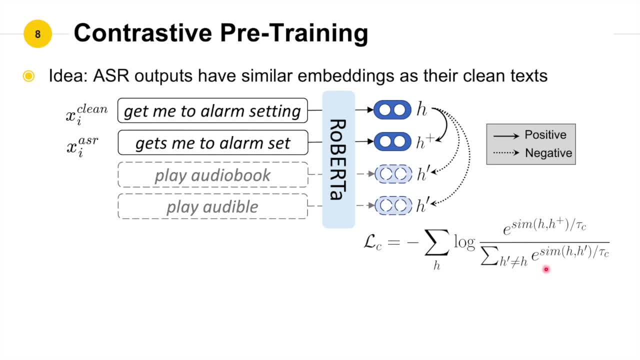 And in the denominator we ask the model to push away the similarity of the negative pairs. So our pre-training objective is the contrastive loss plus the natural language model objective. We keep the MLM loss to prevent catastrophic forgetting and to adapt the model to spoken language. 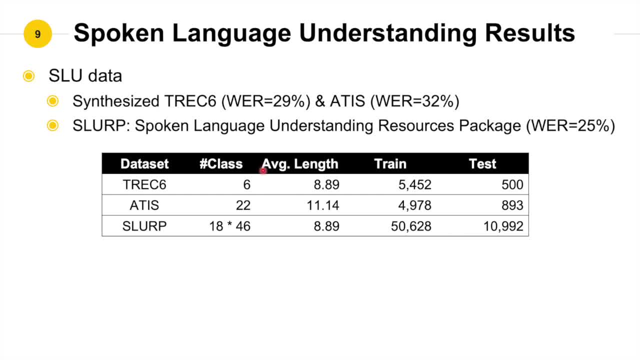 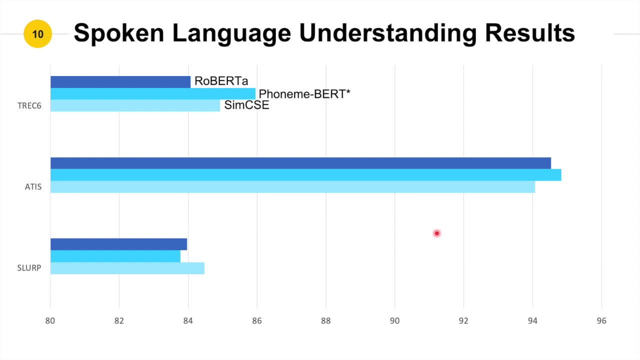 And we verify our result based on three datasets. Track 6 and 8is are the synthesized version with wear rate around 30%. Slurp is another challenging SLU corpus with a wide variety of domains and a larger scale. We compare our method with three baseline models. 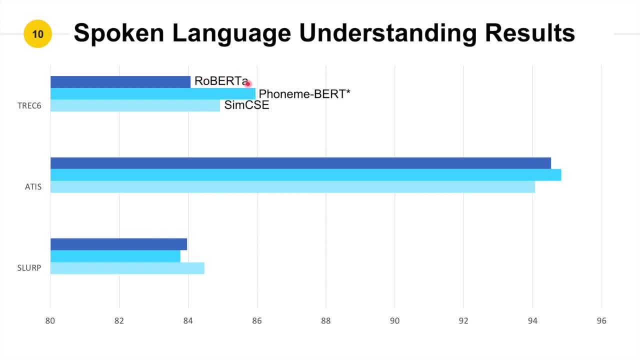 The first one is Roberta, without any modification. The second one is PhonemeBERT, which utilizes additional phoneme sequence and append it after the original text and use the MaxLang model to adapt the pre-trained model. The third one is SimCSE, which is the contrastive learning baseline. 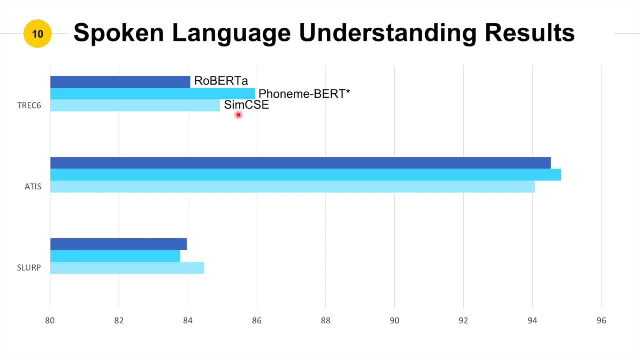 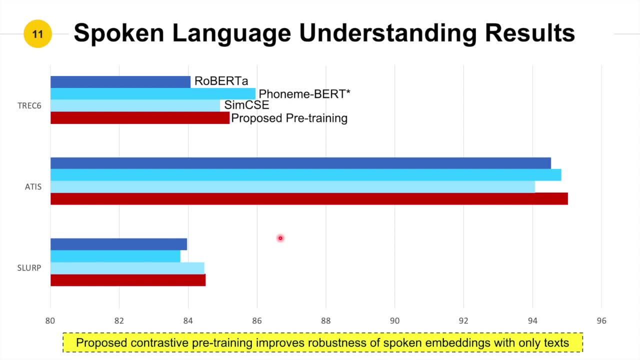 and use two forward passes of the same input source as the positive pair. And here is our result. Our proposed pre-training method have a significant improvement over Roberta across the datasets. We also outperform SimCSE in all datasets by providing additional information of the correct and erroneous text. 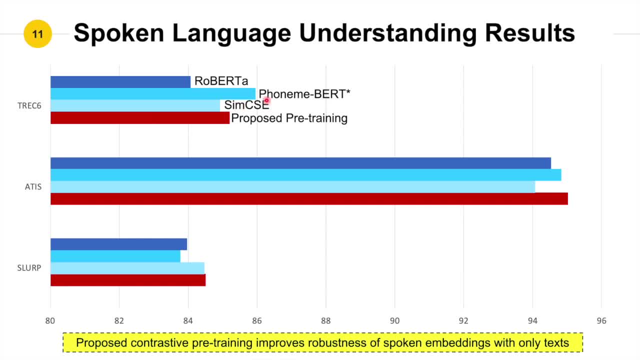 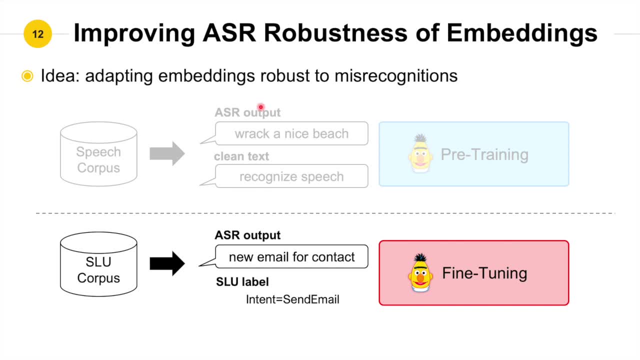 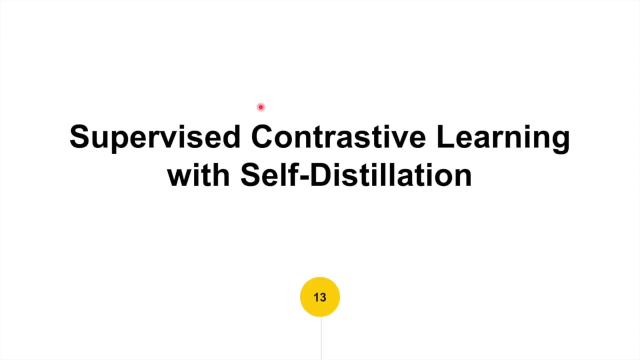 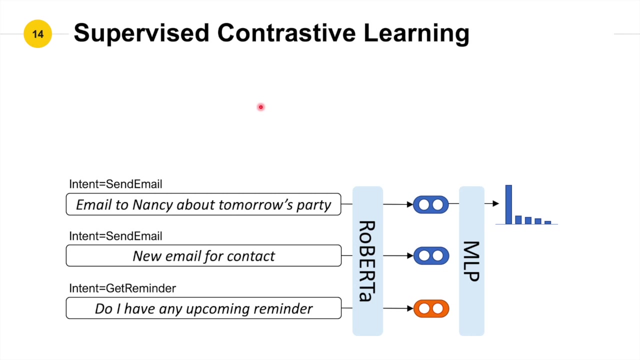 We still lose to PhonemeBERT on track 6,, but they need additional information. Next, let's look at the fine-tuning stage. We propose two techniques to improve the model's robustness to noise. The first one is supervised contrastive learning. 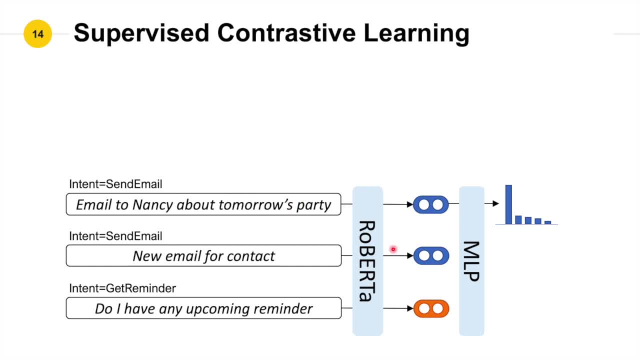 In supervised contrastive learning, the model tries to group together the data with the same label as the positive pair. Like this example, the first two sentences share the same intent- sendEmail- So the model will treat them as positive pair and try to pull together their representation. 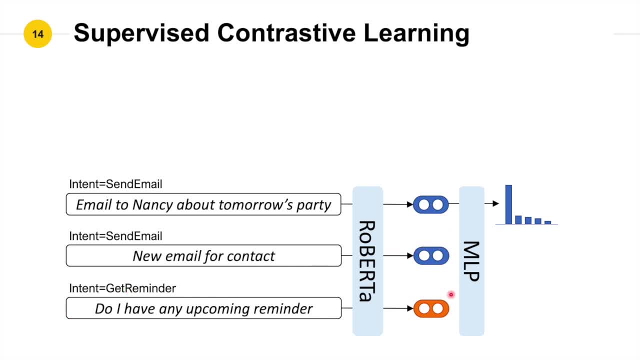 And the third one have a different intent, so the model will try to push away their representation. The idea is that if the data with the same label is very close to each other, then the model will stand a better chance to choose among their representation clusters. 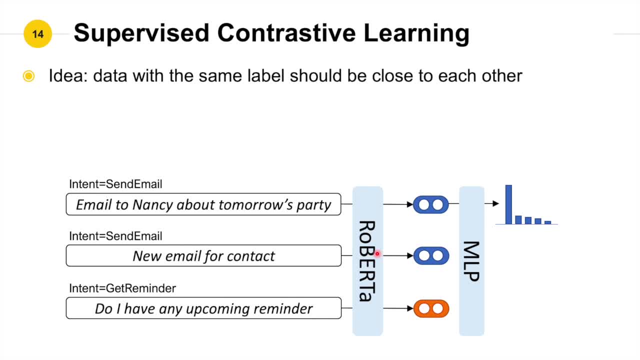 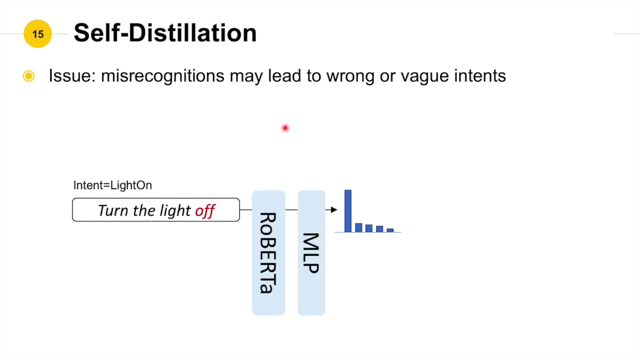 when it sees an input data that is very highly distorted And the objective is written here. It's very similar to the contrastive training, but we add the identity function of the label here to track the positive pairs, And the second one is self-distillation. 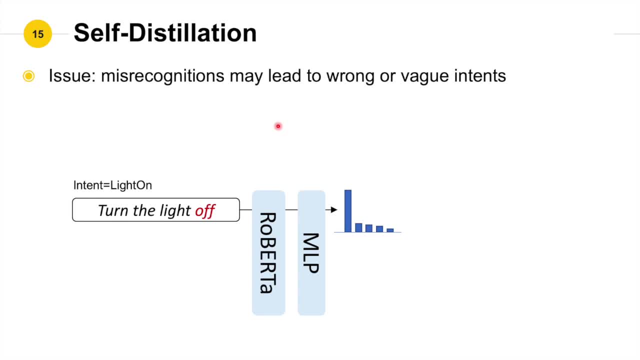 And it aims to relieve the model from label noise. The label noise also comes from misrecognitions put on the keywords, Like this example: the original text should be turned light on, but on is misconscribed to off and the intent is the exact opposite. 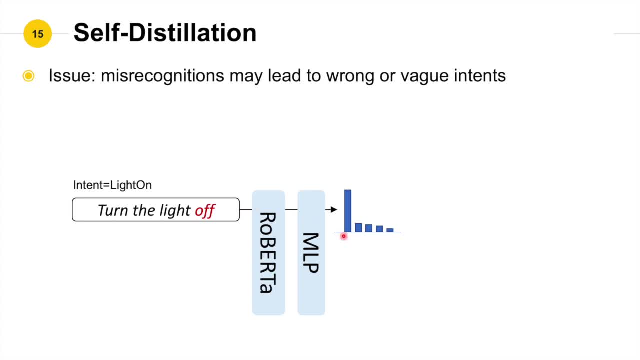 And the model sees this data, it will feel very confused because the intent is very different from the intent. So the model has no choice but to overfit on this misleading label. So we propose to utilize the previous prediction as a guide to check if this label is suspicious. 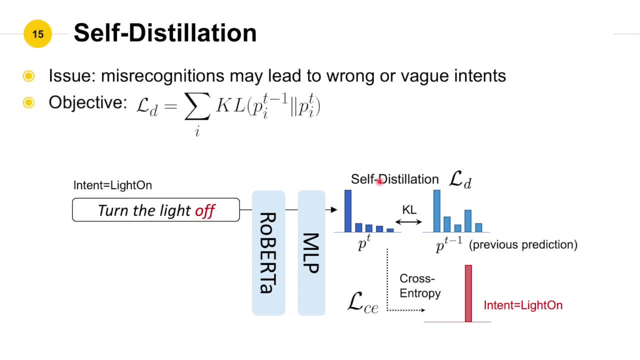 We utilize self-distillation to minimize the KL divergence of the current and the previous prediction so that the model will be more consistent. By this objective, we can force the model not to overfit on the misleading label and therefore reducing the impact of label noise. 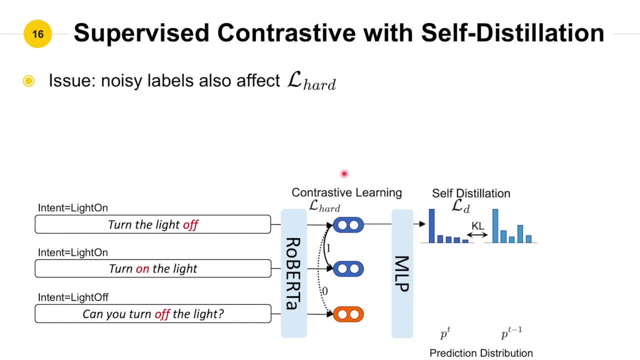 But, as you can imagine, the label problem also affects supervised contrastive learning Like this example: Although the first two sentences share the same label, but since the first sentence is misconscribed, actually the first and the third one has better semantic similarity. 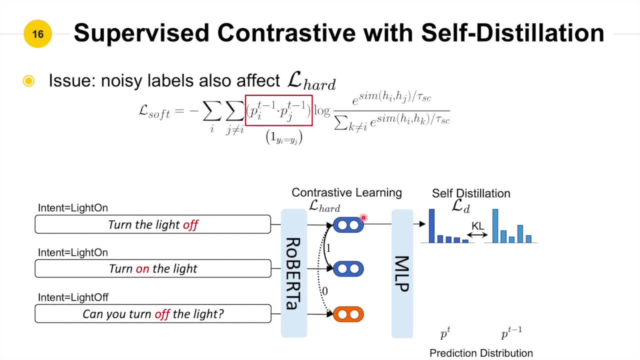 So we replace the identity function in the supervised contrastive learning with the soft label score And the score is calculated by the dot product between the previous prediction, So that the model will know that the first two is actually quite different and the first and the third one is more similar. 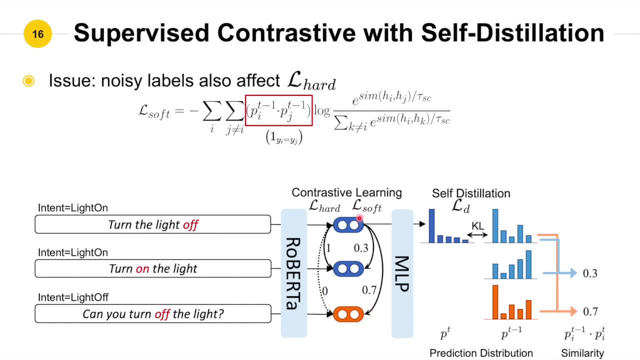 And we use this score as an indication of how the model should try to pull the representation together. So the final fine-tuning objective is the weighted sum of the cross-entropy loss, the self-distillation KL divergence and the hard-label and soft-label version of supervised contrastive learning. 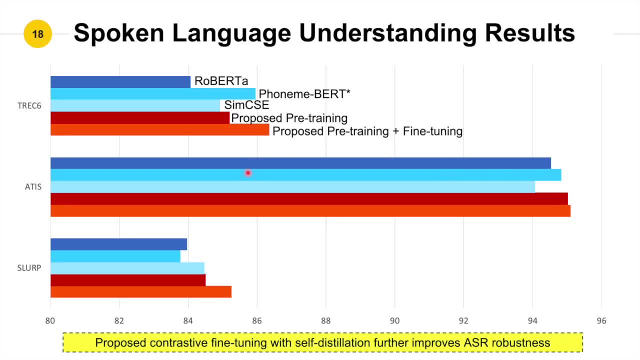 And here is our result. The proposed fine-tuning method further boosts the performance across the dataset And we even outperform falling birds on track 6.. Although the improvement on ATIS is relatively small, it's mainly because of the label noise in the test set. 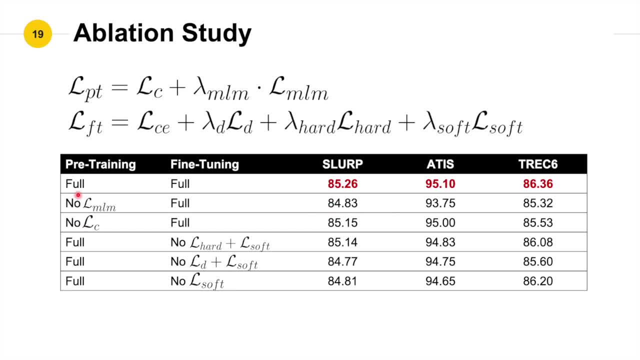 And here is our ablation study. The first two rows are for the training stage and the later three rows are for the fine-tuning stage. We can see that in the pre-training the masked language modeling is very important to adapt the model to spoken language. 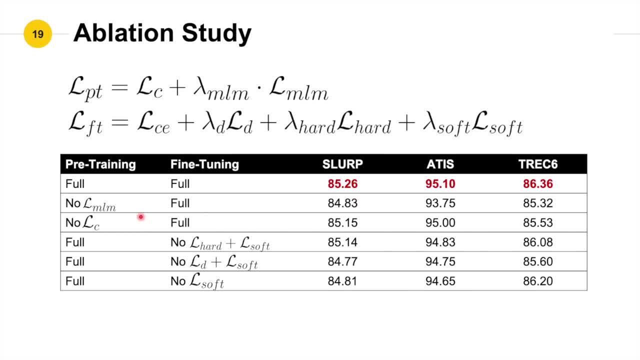 and prevent catastrophic forgetting. when we applied the contrastive loss In the fine-tuning stage. we can see that the self-distillation is very important to prevent the model from overfitting the misleading labels. Overall, we can see that each component contributes positively to the final score. 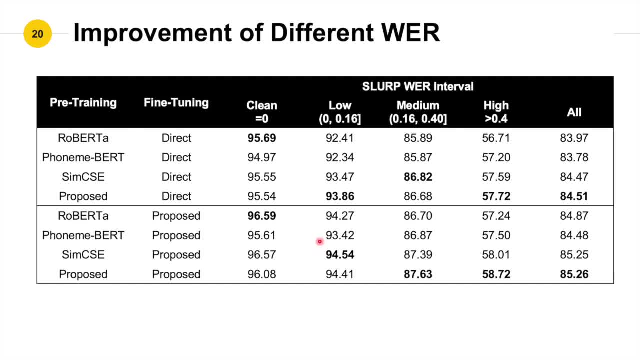 In the last section. let's check which part of the data actually improved. We can see the column stands for data with different reiterate intervals. The first one, the first column, does not contain any error And it turns out that the Roburda base is the best model. 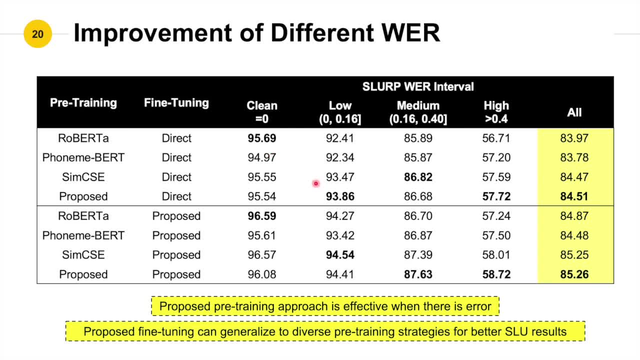 However, as long as there is a recognition error in the input data, our proposed pre-training method provides a significant improvement And we can look at the four later rows which uses the proposed fine-tuning techniques. We can see that the performance is improved.